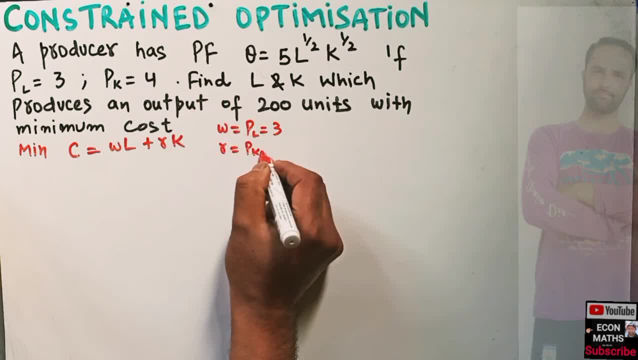 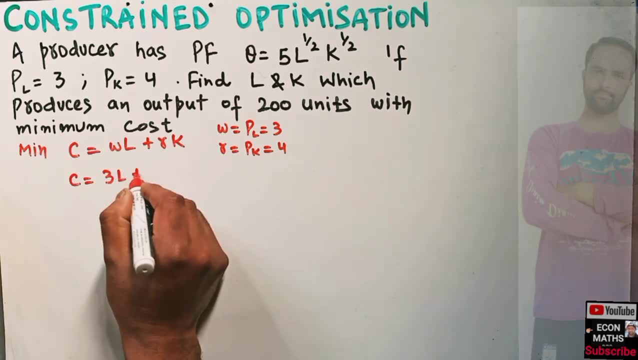 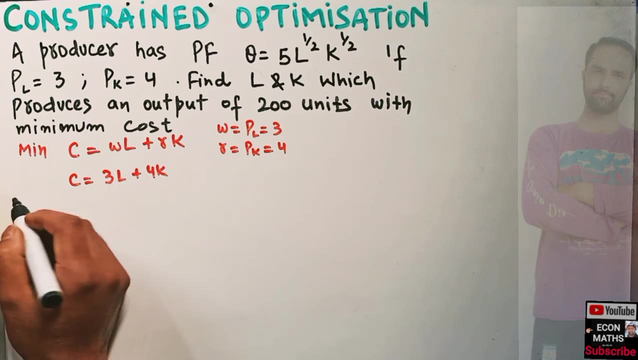 Rental rate of capital is price of capital which is being given us here, 4.. That means we want to minimize this. C is equal to 3L plus 4K. Okay, we want to minimize our cost, given the production constraint. And what is our production constraint? This, that is, 5L to the power 1 upon 2 times K to the power 1 upon 2, should be the cost of labor. 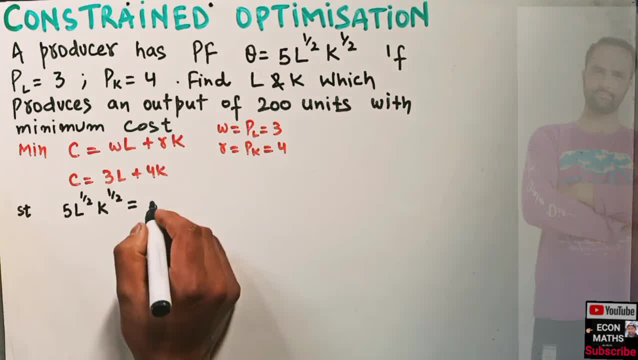 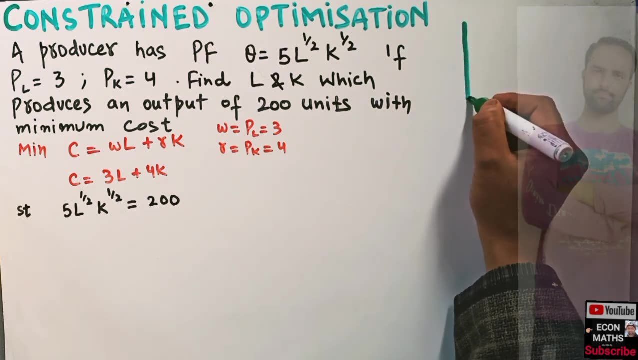 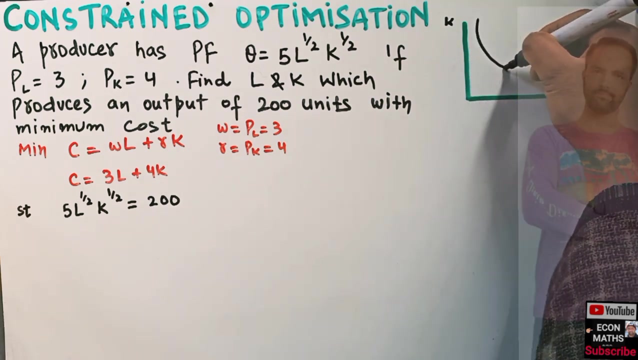 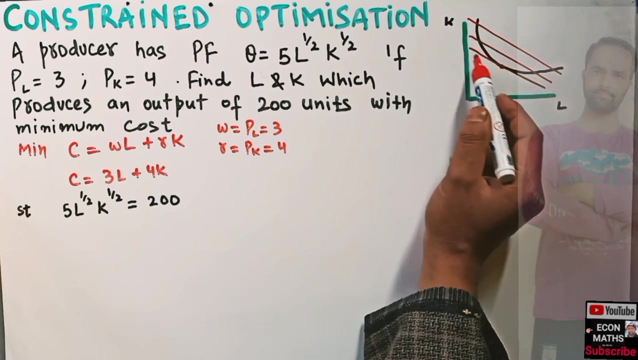 And what is our production constraint? This, that is, 5L to the power 1 upon 2 times K to the power 1 upon 2, should be the cost of labor. Let us say we are being given the Cobb Douglas production function here, And let me use another color. Let us say we are being given this production function. We want to achieve this production quota with minimum cost. That means we want to minimize our cost in such a way- And cost will be minimized when this, the slope of the production function, is equal to 3L. 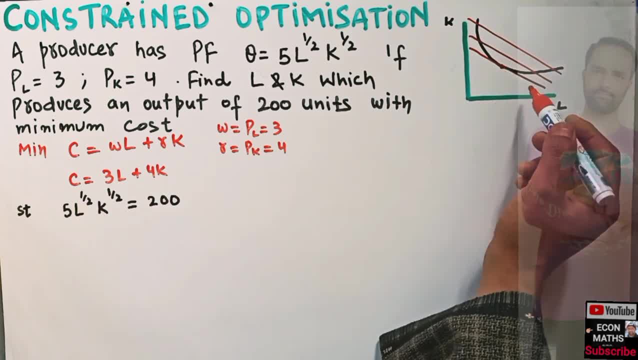 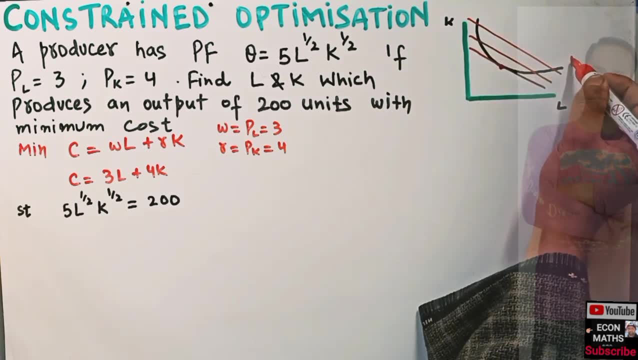 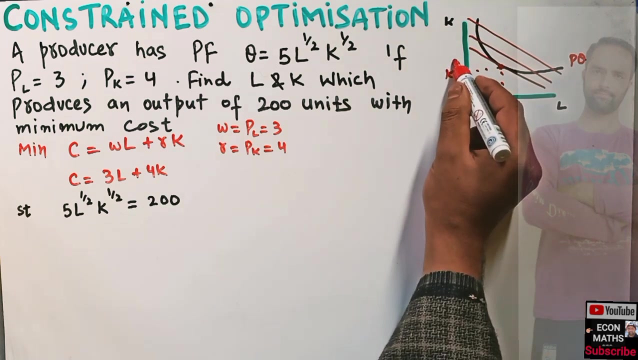 Let us say we are being given the Cobb Douglas production function here, And let me use another color. Let us say we are being given this production function here And cost will be minimized when this- the slope of the production function, is equal to 3L. 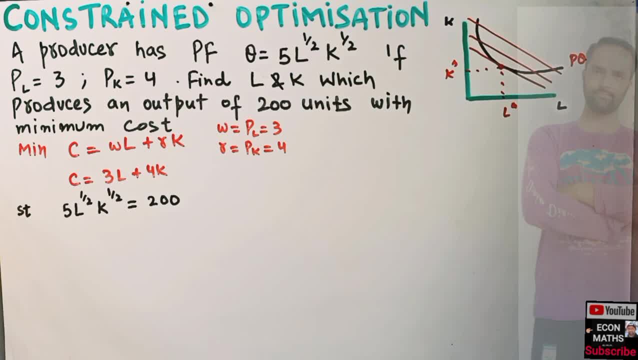 Let us say we are being given this production constraint here, And cost will be minimized when this the slope of the production function is equal to 3L. Let us say we are being given this production constraint here And cost will be minimized when this the slope of the production function is equal to 3L. 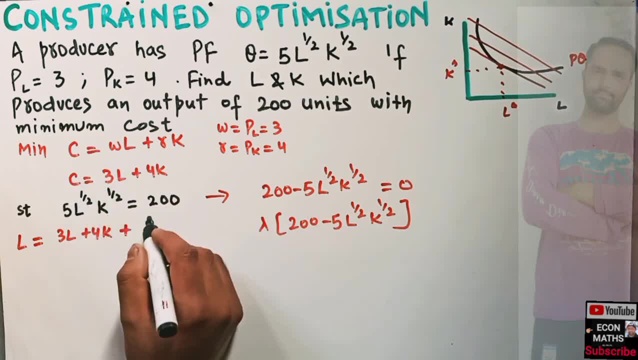 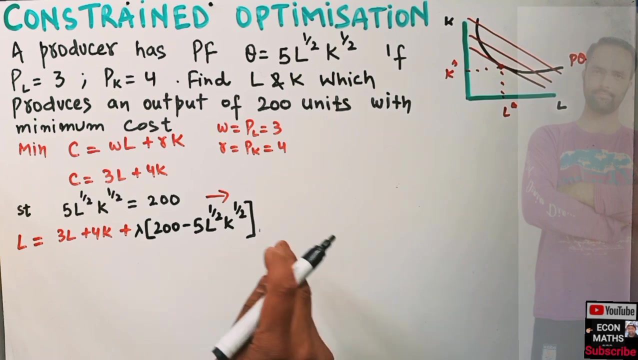 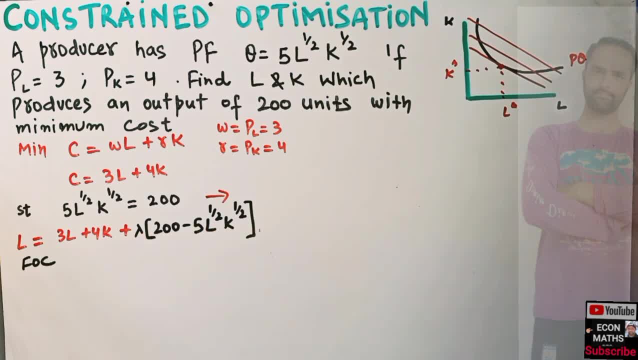 Let us say we are being given this production constraint here And cost will be minimized when this, the slope of the production function, is equal to 3L them simultaneously and that exactly means we need to find the L subscript. L that mean is partial derivative of this function with respect to labor derivative. 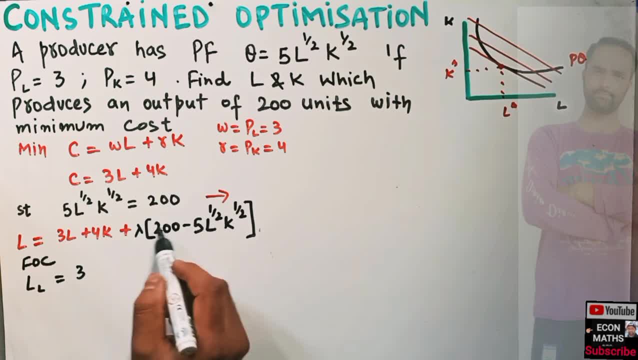 of L is 1, so we are left with 3 here. derivative of L will be L to the power 1 upon 2 we have. it will become 1 upon 2. L to the power minus 1 upon 2. okay, so we will get here minus for you, for you, into 1 upon 2. L to the power minus 1 upon 2 K. 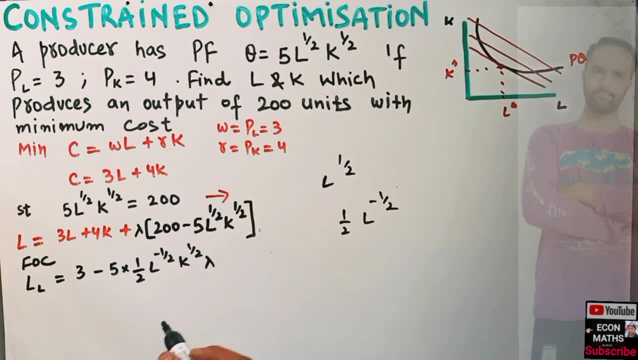 to the power 1 upon 2 and we have the lambda. you can see, if I take the partial derivative of this function with respect to labor, I will get this stuff symmetrically taking partial derivative of the Lagrange's function with respect to capital. this time derivative of K is here 1, so we are left with 4. then we 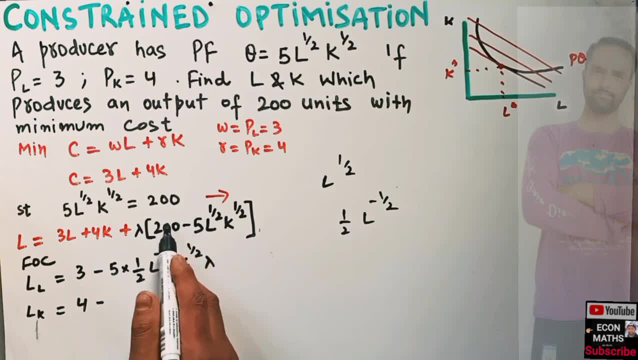 have minus again day. it is constant, it is. your derivative is 0, so we will again get minus for you into 1 upon 2, since we are taking derivative with respect to K. so we will have K to the power minus 1 upon 2 and L to the power 1 upon 2 will. 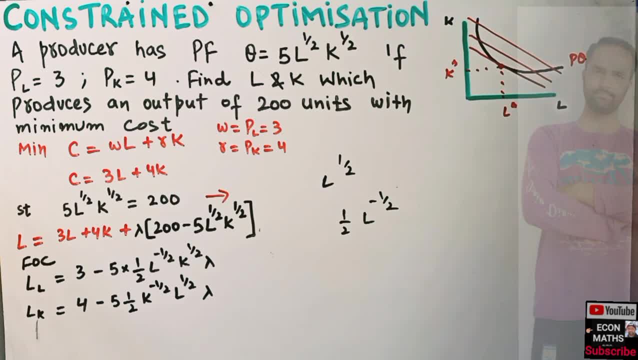 remain same and we have the lambda here. okay, so we less be the derivative forWell, so we take only 2, we don't need dragging the derivative with respect to lambda here. okay, so we will solve these two equations. first, we set it equal to 0, this also equal to 0, and 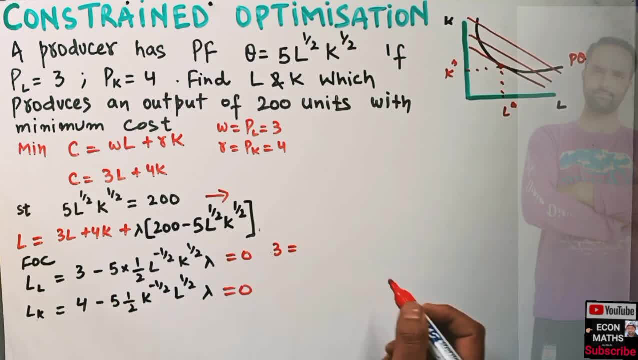 if we rewrite these two equations, I can write it in this fashion: that is: 3 is equal to transposing here. it will become for you: upon 2 L to the power minus 1 upon 2 K to the power 1 upon 2 lambda and 2 Land1, it will use in prediction 25 grand per second. so this is our equationions that I added here. 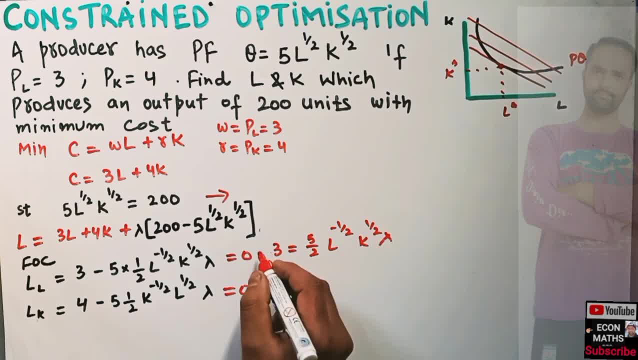 This equation implies: 4 is equal to 5 upon 2, k to the power minus 1 upon 2, l to the power 1 upon 2 lambda. okay, Now let's divide these two equations, So dividing here LHS with LHS and RHS with RHS, okay. 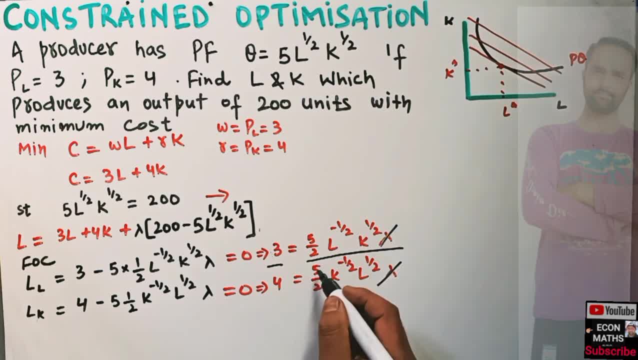 So we have these two equations: Lambda, lambda gets cancelled, 5 upon 2, 5 upon 2 gets cancelled, okay. So what we get here? If I transpose this k to the power minus 1 upon 2 to the numerator, its exponent sign will get changed, okay. 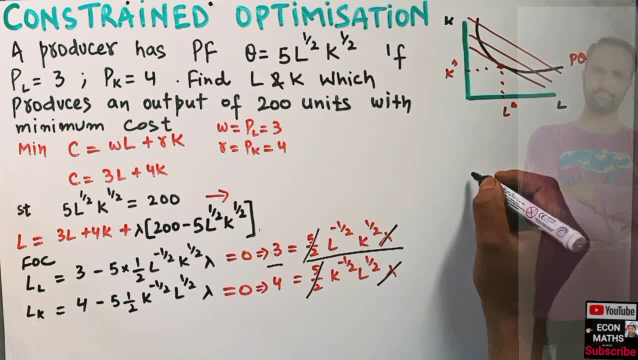 So it will get multiplied with this k to the power 1 upon 2.. Simple thing: we have k to the power 1 upon 2 in the numerator, k to the power minus 1 upon 2 in denominator. I can write this in this fashion: 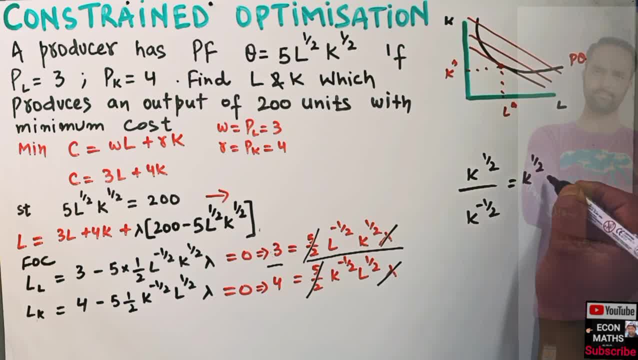 And that means k to the power 1 upon 2.. Transposing this, it will get multiplied and exponent sign changes. It becomes 1 upon 2, okay, So, which implies 3 upon 4 is equal to k to the power 1 upon 2, k to the power 1 upon 2.. 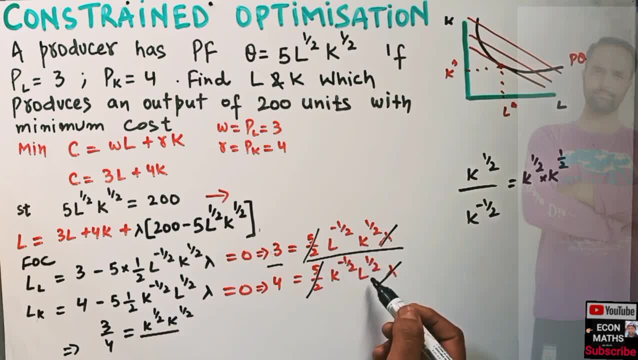 Symmetrically. if I transpose this L to the power minus 1 upon 2 to denominator, it will get multiplied with this L and exponent sign will change And we will get L to the power 1 upon 2.. And we will get L to the power 1 upon 2.. 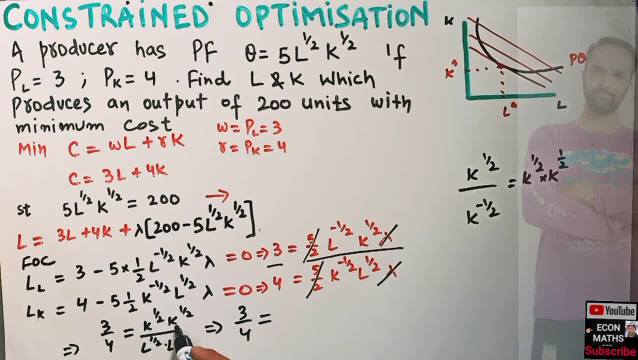 Which implies 3 upon 4 is equal to. bases are same, powers can be added, So 1 upon 2, 1 upon 2 becomes 1.. So we are left with k upon L, Which implies k is equal to 3 upon 4 L. okay. 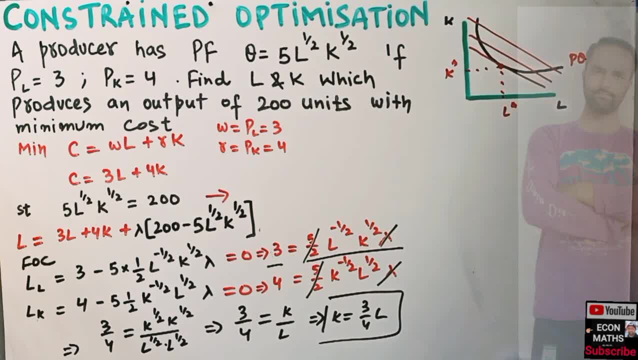 Okay, Now what we do? We simply put the value of k is equal to 3 upon 4. Is equal to L into this equation, in this production quota. That means we have 5 L to the power, 1 upon 2, k to the in place of k. we have this stuff. 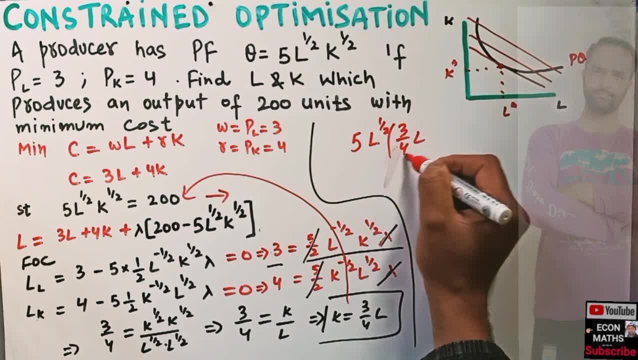 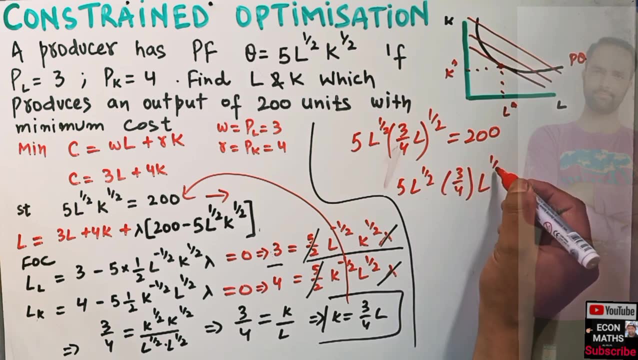 That is 3 upon 4. L to the power 1 upon 2 is equal to 200.. So we will get 5 L to the power 1 upon 2.. We have 3 upon 4.. L to the power 1 upon 2 is equal to 200.. 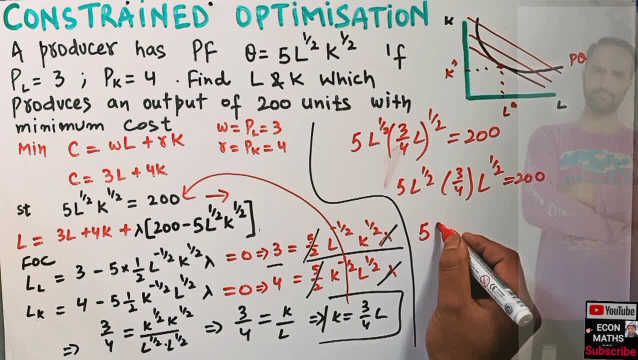 L to the power 1 upon 2,. L to the power 1 upon 2,, it will become 5 L. Bases are same exponents add up to 1. Here it is 1 upon 2.. Okay. 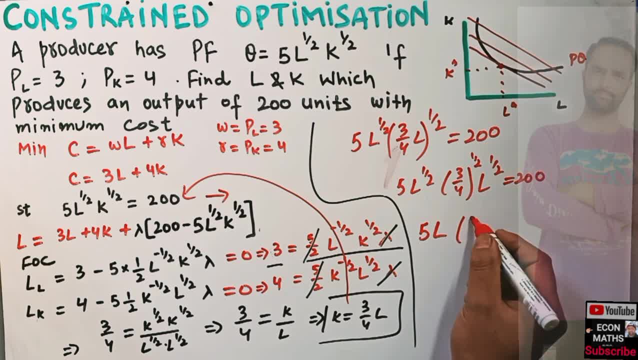 So 5, L, 3 upon 4, 1 upon 2 is equal to 200.. Which gives us L is equal to Okay. It will become 200.. Transposing it will become 5.. If I transpose, it will get reciprocated and it will become, under root, 4 upon 3 here.